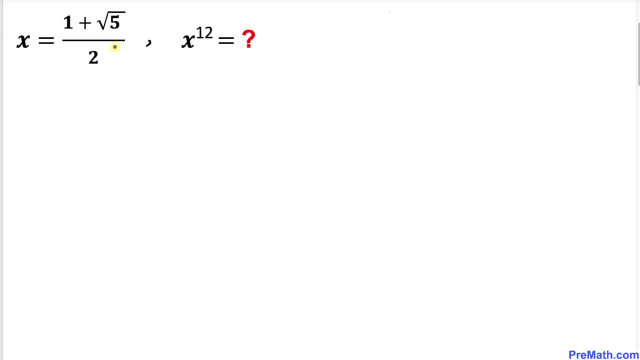 thumbs up to this video. So let's go ahead and get started with the solution, and here's the very first thing we are going to do. Let's focus on this golden ratio, and here I have copied it down as you can see. Let me go ahead and make it a fraction on the left hand side by just putting. 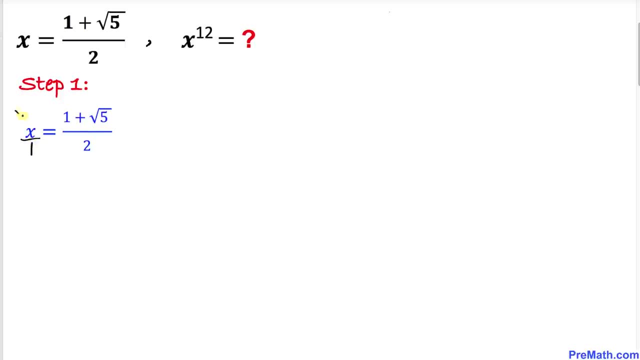 1 underneath this x, and now we are going to cross multiply, and if we cross multiply, we are going to get 2x equals to 1 plus square root of 5.. We are going to isolate this radical part, so therefore, I'm going to move this one on the 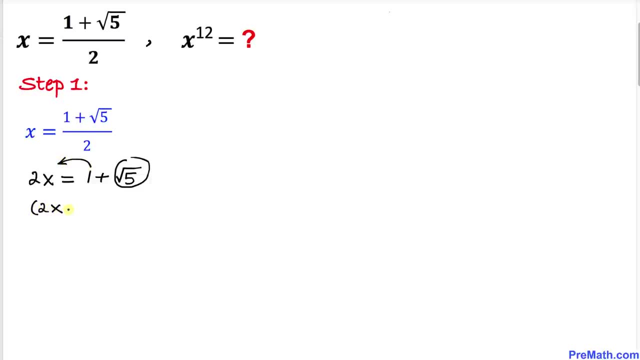 other side. so this is going to become: 2x minus 1 equals to square root of 5. and now let's take square on both side: power 2 on this side and power 2 on this side as well. and now we are going to use: 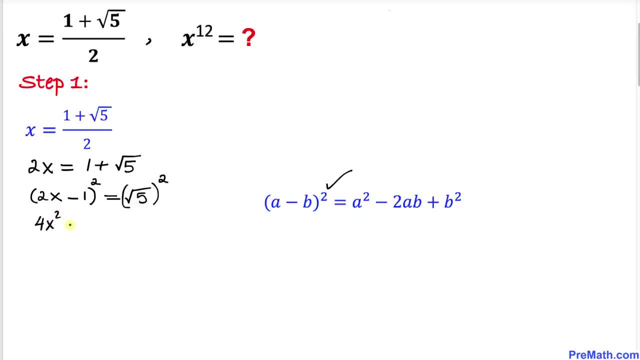 square root of 5.. So this could be written as: 4x square minus 4x plus 1 equals to this square and square root. they undo each other. we simply ended up with 5.. Now let's go ahead and subtract 5 from: 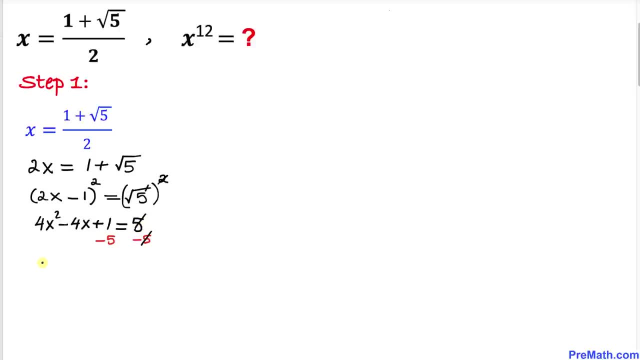 both side, this 5 and negative 5. they are gone, so we ended up with 4x square minus 4x minus 4, equal to 0.. Now we can see that each and every term is divisible by 4, so I can divide by 4 across. 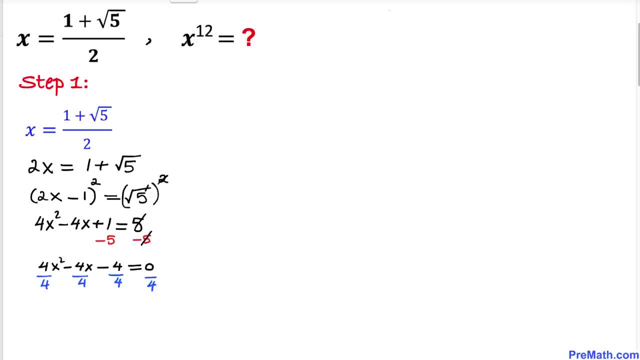 the board. so we simply ended up with this 4, and 4 is gone with this thing. so we ended up with x square. so same thing over here: negative x, and that is going to give us negative 1 to 0.. Now we want to isolate x square. I'm going to remove these x, negative x and negative 1 on. 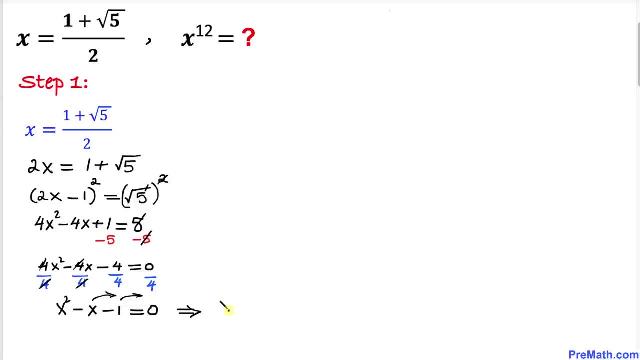 the other side. so that means we are going to have x square becomes x plus 1, and now let me go ahead and call this as an equation number 1. and here's our next step. let's focus on this: x power 12. we are going to manipulate. 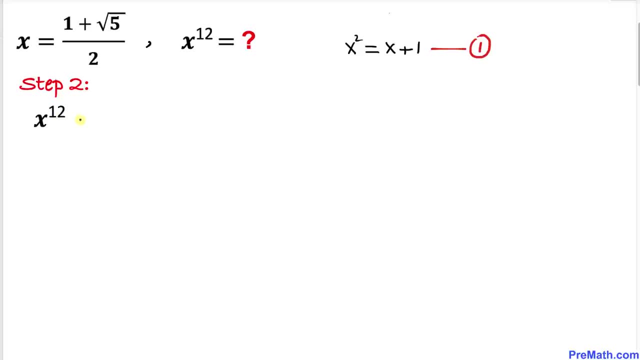 this one, and here I have copied down x power 12, and this could be written as x power 2 and then power 6, because we can write as a nested exponent. and now let's focus on this x square. I am going to replace it by this x plus 1 from this equation 1, so this could be written as x plus 1 and then. 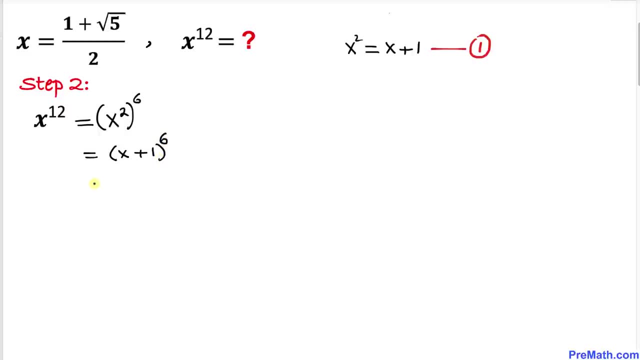 power 6. and now, once again, we are going to tweak this thing. I can write this x plus 1, power 6 as x plus 1 square, and then power 3. and now let's go ahead and apply this a plus B square formula to expand this binomial, so this could be written as a x square plus 2x, and then a plus one, and then 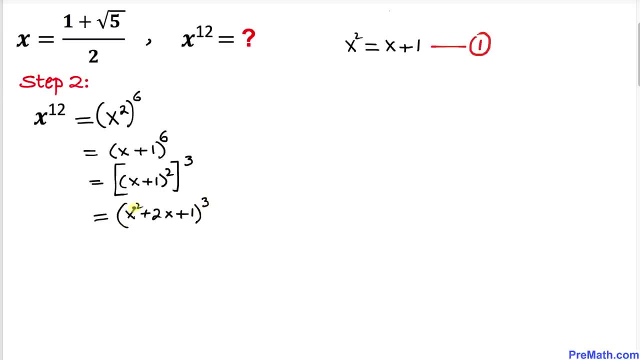 then whole power 3, and now, once again, wherever we see x square, i am going to replace it by x plus 1 from this equation 1, so therefore, this could be written as x plus 1, and then i'm going to leave these one as it is: plus 2x plus 1, and then power 3, and this, in turns, could be written as: 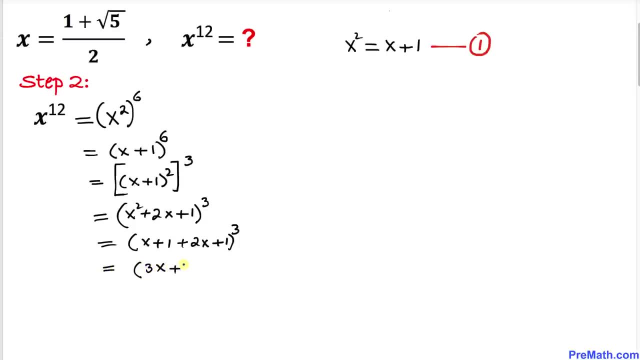 3x plus 2, whole power 3, and now this could be written, as if we tweak it a little bit: 3x plus 2, power 2, and then 3x plus 2, power 1, and now let's use this formula once again: 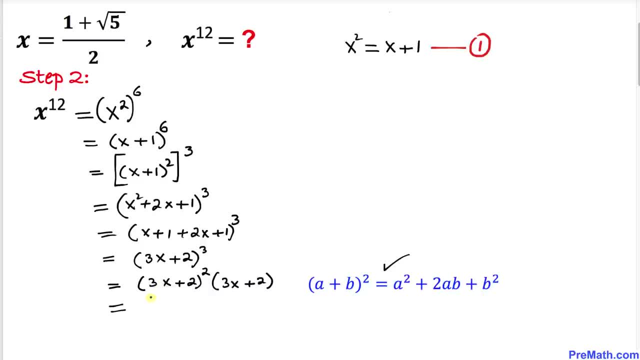 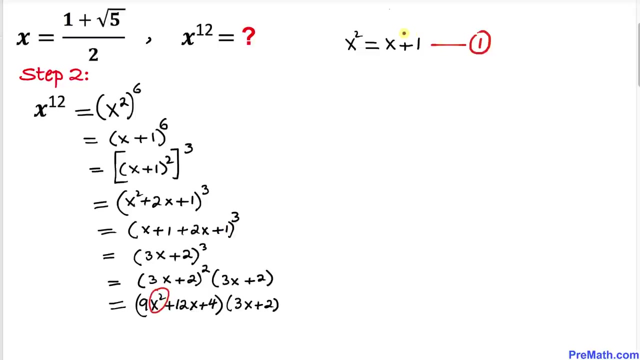 so the left hand side. this part is going to be written as 9x square plus 12x plus 4 and then times. i'm going to leave this one as it is 3x plus 2. now we can see that x square once again showed up, so i am going to replace it by x plus 1 from. 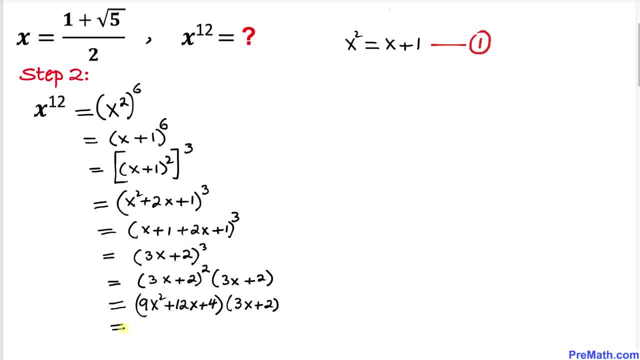 this equation 1, so this could be written as 9 times x plus 1, and then plus 12x plus 4, and then times 3x plus 2, and in this next step i have just distributed this 9, so this becomes 9x plus 9, and then 12x plus 4, and i left everything same as it is. and on the 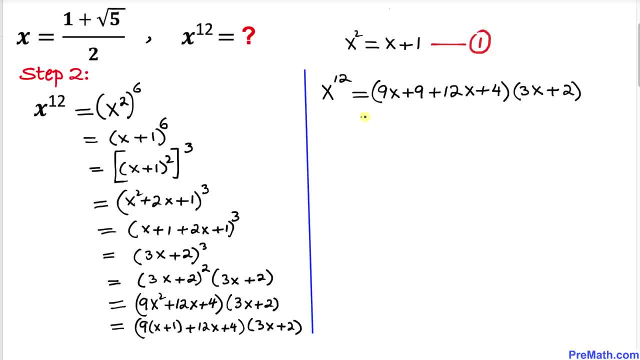 left hand side. we got x power 12, and now let's go ahead and combine the like terms, so we got 21x plus 13 times 3x plus 2. now let's go ahead and multiply these two binomials by using a double distribution, so we are going to get 63x square plus 42x plus 39x. 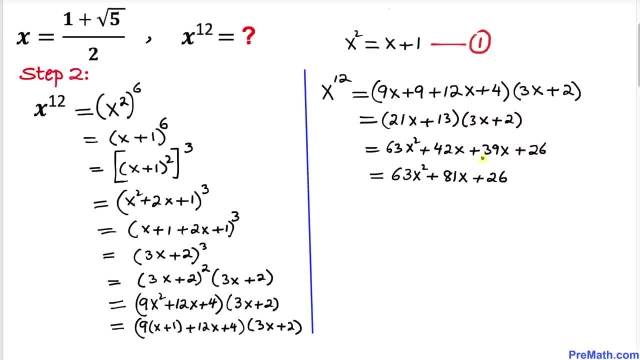 plus 26, and here, in this next step, i have combined these two like terms and we got 81x. now we can see that once again, this x square showed up, so i'm going to replace it by x plus 1 once again, so this could be written as 63 times x plus 1 plus everything is going to be same: 81x plus. 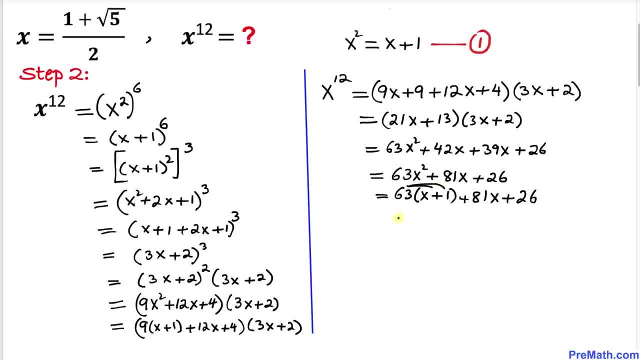 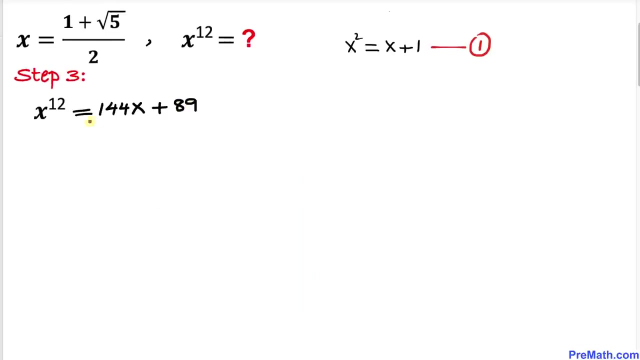 26. let's go ahead and distribute these ones. so we are going to get 63x plus 63 plus 81x plus 26. so if we combine the like terms on the right hand side, we are going to get 144x plus 89. so finally we got x power. 12 equals to 144x plus 89. and now we are going to replace: 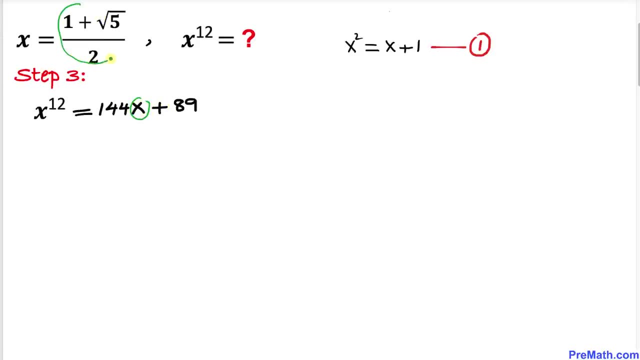 this x by this fraction: 1 plus square root of 5 divided by 2, so let's go ahead and replace that one. so 144 times here i'm gonna write down 1 plus square root of 5 divided by 2, and then plus.